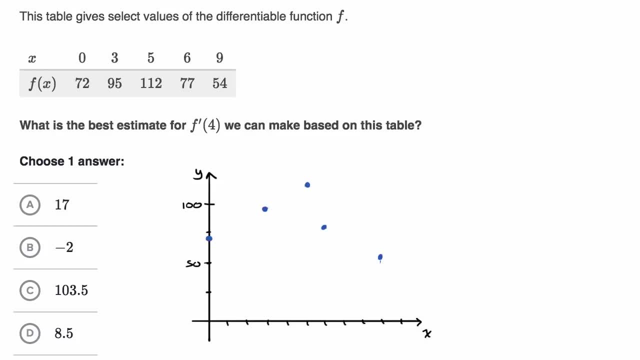 We know that these would sit on the curve: of y is equal to f of x. When x is zero, f of x is 72.. So this is the point zero, 72.. This is the point three comma 95.. 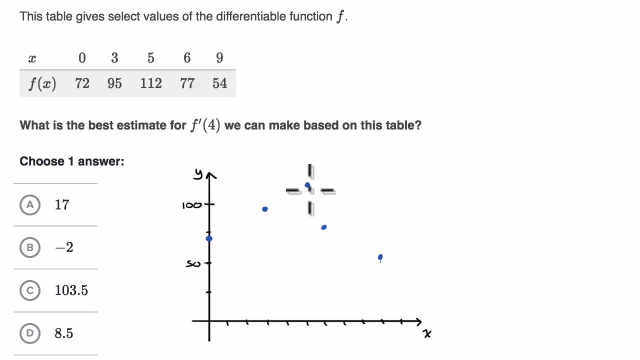 Clearly two different scales on the x and y axis. This is the point five: 112.. This is 677.. This is 954.. Actually, let me write out the. this is one, two, three, four, five, six. 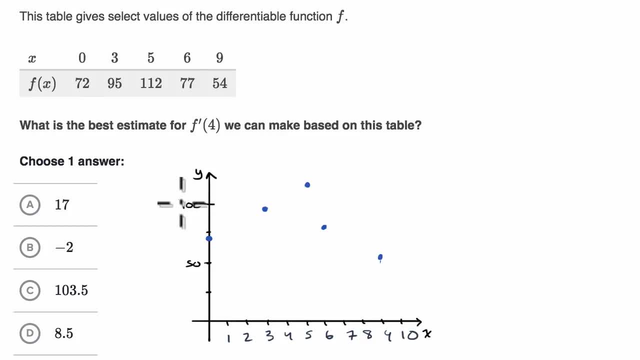 seven, eight, nine and 10.. Now they want us to know. they wanna know what is the derivative of our function when f is equal to four. Well, they haven't told us even what the value of f is at four. 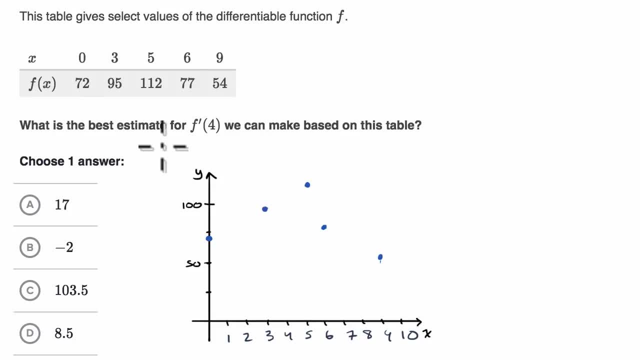 We don't know what that point is, But what they're trying to do is, well, we're trying to make a best estimate And, using these points, we don't even know exactly what the curve looks like. It could look like all sorts of things. 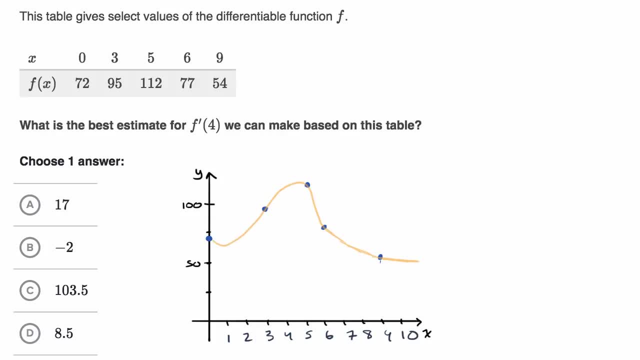 We could try to fit a reasonably smooth curve. The curve might look something like that, But it might be wackier. It might do something like this. Well, let me try to do it. It might look something like this, So we don't know for sure. 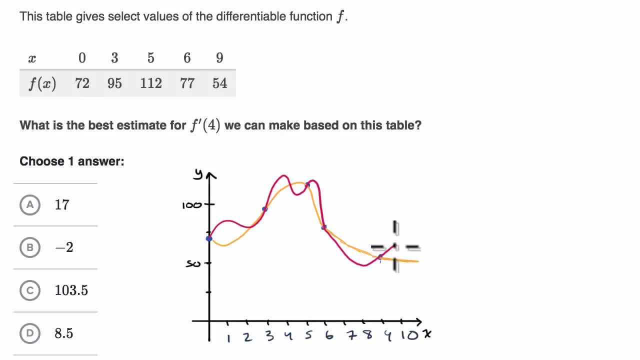 All we know is that it needs to go through those points because they've just sampled the function at those points. But let's just for the sake of this exercise, let's assume the simplest. let's say it's a nice, smooth curve. 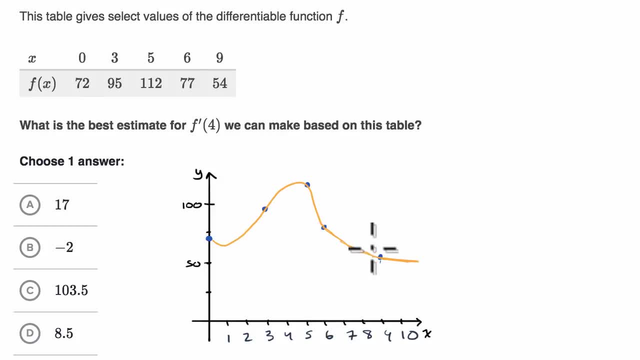 without too many twists and turns. that goes through these points just like that. So what they're asking? okay, when x is equal to four, if this yellow curve were the actual curve, then what is the slope of the tangent line at that point? 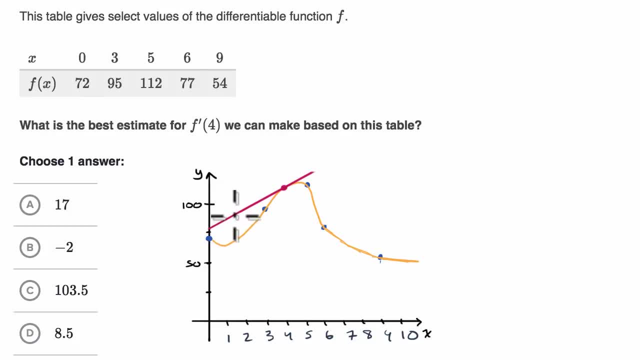 So we would be visualizing that. Now, to be clear, this tangent line that I just drew, this would be for this version of our function that I did connecting these points. That does not have to be the actual function. We know that. the actual function 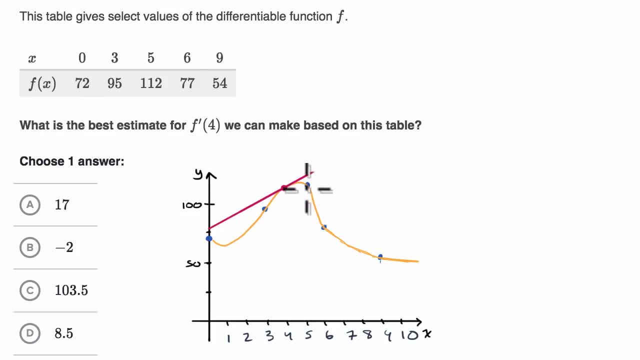 has to go through those points. but I'm just doing this for visualization purposes. One of the whole ideas here is that all we do have is a sample and we're trying to get a best estimate. We don't know if it's even gonna be a good estimate. 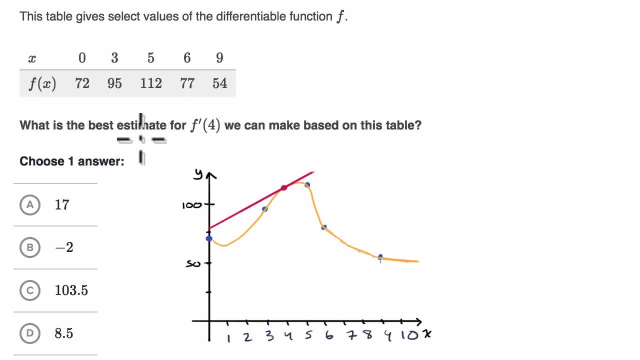 It's just going to be a best estimate. So what we generally do when we just have some data around a point is let's use the data points that are closest to that point and find slopes of C decant lines pretty close around that point. 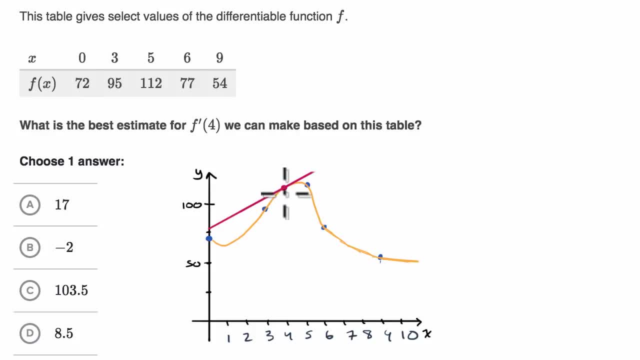 and that's going to give us our best estimate for the slope of the tangent line. So what points do we have near f of four, or near the point four, comma f of four? Well, they give us what f is equal to when x is equal to three. 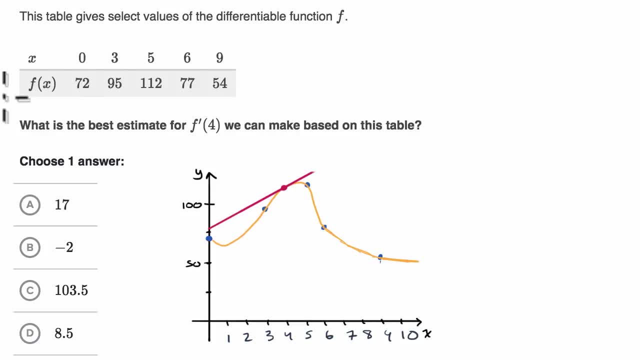 They give us this point right over here- Let me do this in another color- So three comma 95, that is that right over there. and they also give us five comma 112.. That is that point right over there. and so what we could do, we could say: 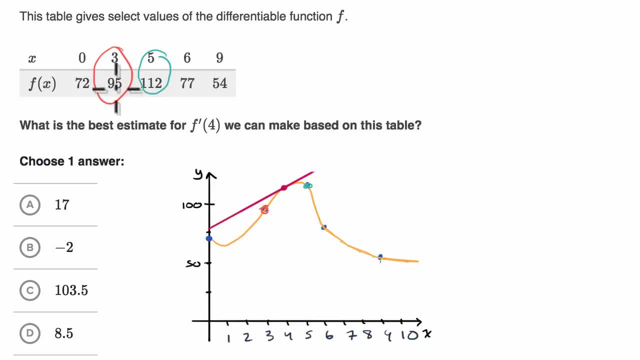 well, what is the average rate of change between these two points? Another way to think about it is: what is the slope of the secant line between those two points? and that would be our best estimate for the slope of the tangent line at x equals four. 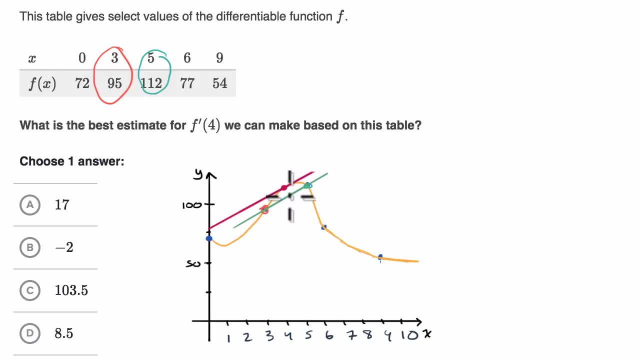 Do we know that it's a good estimate? Do we know that it's even close? No, we don't know for sure, but that would be the best estimate. It would be better than trying to take the average rate of change between when x equals three and x equals six. 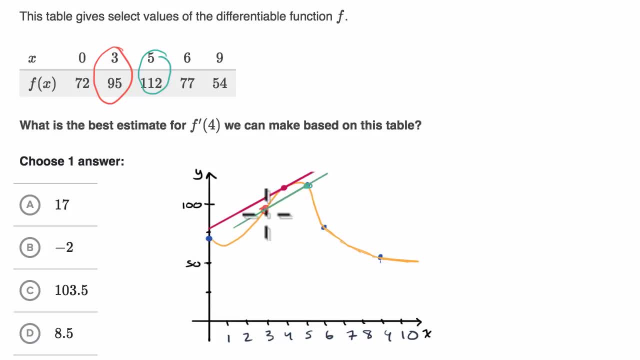 and when x equals zero and x equals nine. These are pretty close around four, and so let's do that. Let's find the average rate of change between when x goes from three to five. So we can see here our change in x. 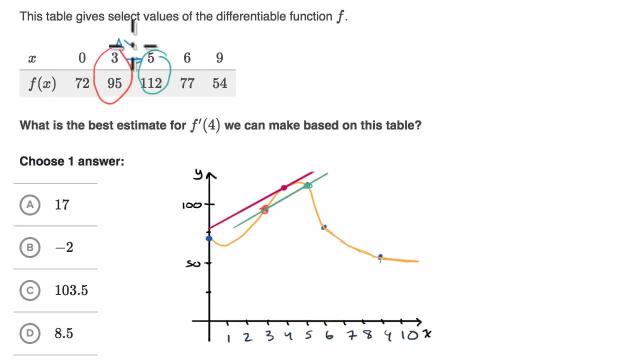 let me do this in a new color. So our change in x here is equal to plus two, and I can draw that out. My change in x here is plus two and my change in y is going to be when my x increased by two. 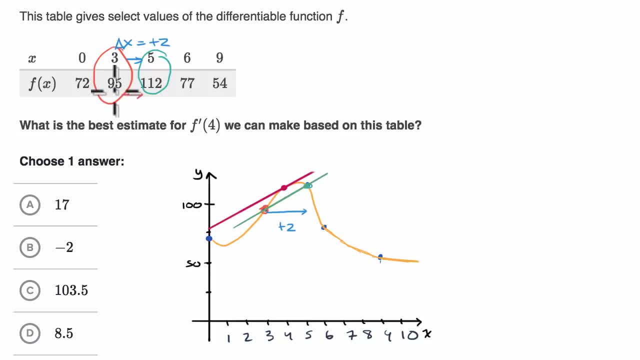 my change in y is plus. let's see this is, if I add 10, I get to 105, and then I add another seven. so this is plus 17.. So this is plus 17, right over here, Plus 17..